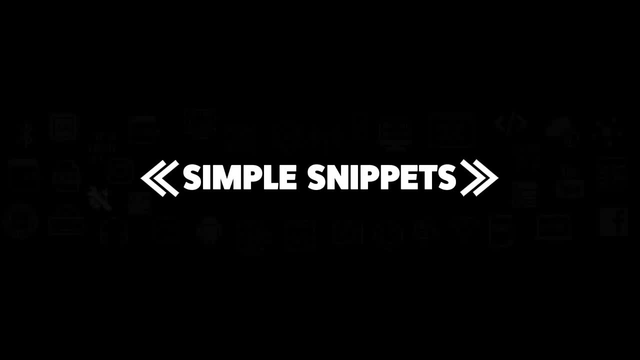 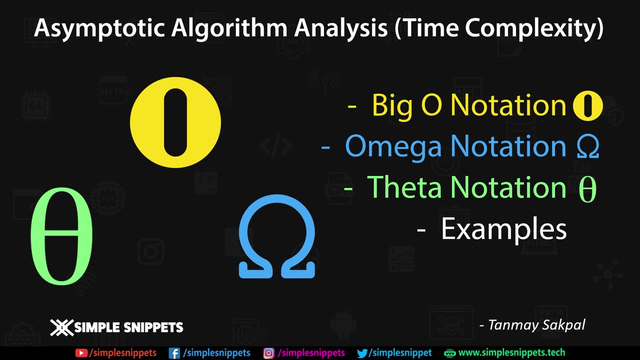 Yo, what's going on guys? Tanmay here for Simple Snippets and welcome back to another video tutorial on Data Structures and Algorithms, and this is a second topic on algorithm analysis, wherein we are gonna be taking a detailed look at the three different types of time. 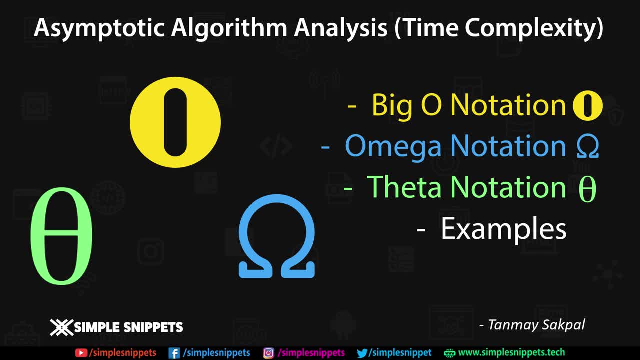 complexities and the three different types of analysis that we do, which are denoted by these three different notations, as you can see on the screen: the big O notation, the omega notation and the theta notation. Now, before we start off with this tutorial, 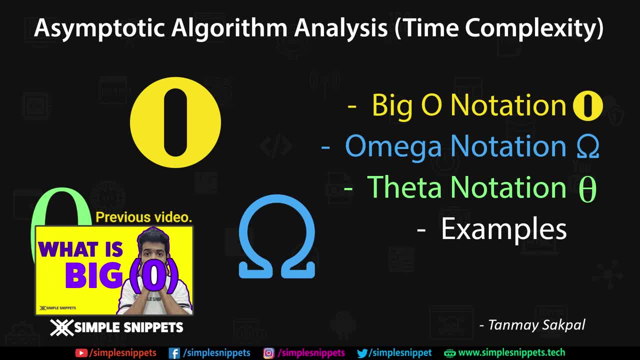 if you don't know what algorithm analysis is or why do we need algorithm analysis, make sure you watch the previous video in this Data Structures playlist. If you want, I'll link that video in the video description or you can also see a card on the top right corner. 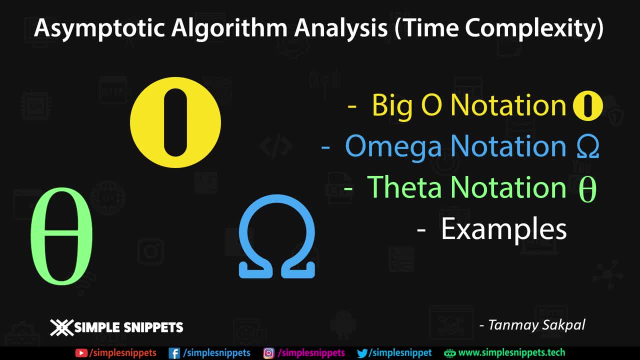 because in that video we took a very detailed understanding of what is algorithm analysis, what is asymptotic algorithm analysis? why do we need it? We also saw what is big O notation and how we can calculate the big O notation ourselves. So if you are not really sure, 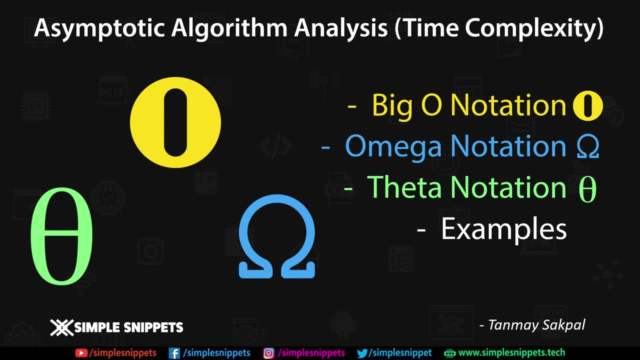 about this entire algorithm analysis topic. just make sure you watch that video. That will clear out many of your doubts. and if you are only particularly looking for the three different types of time complexities, then this video is just for you. Make sure you watch this video till the end and everything will be very clear. So, with that being said, 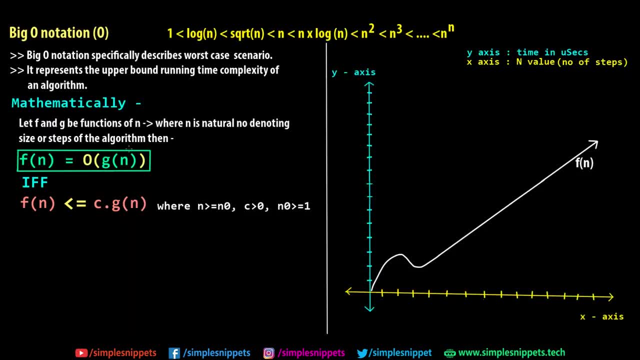 let's get started. So let's start off with the very first type of algorithm analysis, that is, the big O notation. and starting off, the big O notation specifically describes worst case scenario, so it represents the upper bound running time complexity of an algorithm. so what does this mean? so on this right hand side, you can see, we have a graph. on the x-axis, we have 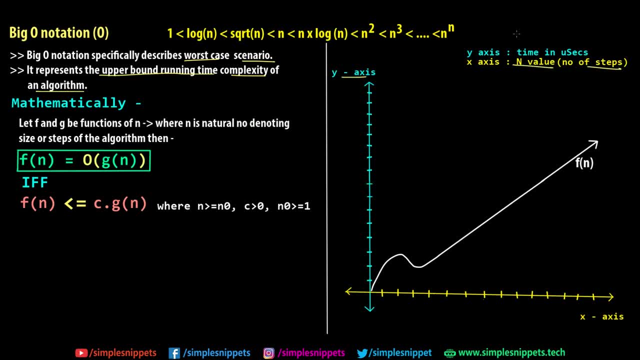 n value, which is basically the number of steps, and the y value is, or the y-axis is the time in microseconds or any units of time. okay, so whenever an algorithm is running, obviously it will take some amount of time, and algorithm analysis, in a nutshell, is basically us trying to find out that. 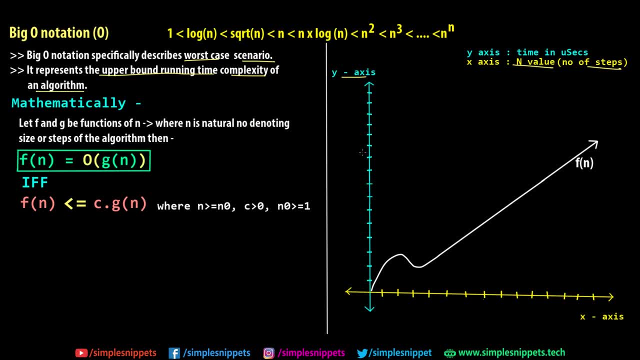 behavior, as to how the algorithm behaves, basically in terms of time given a certain input. so, for example, if the algorithm requires 10 steps and it is taking 10 seconds, this is just an example. what happens when those 10 steps are multiplied by 2? what happens when we have 20 steps? then what? 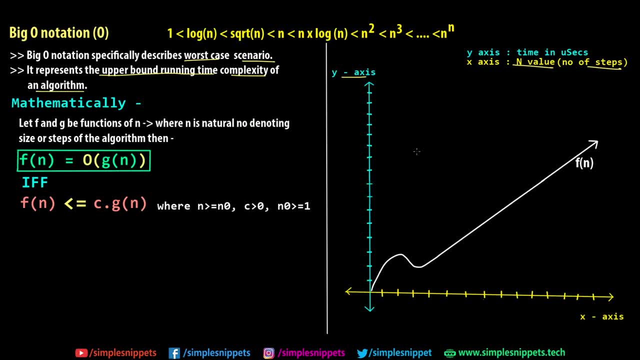 is the time taken. is it 20, which means it would be a linear time. basically, this graph is actually showing a linear time scenario only so you can see as the n value increases. so n is basically the number of steps it can be taken as the number of steps it can be taken as the number of steps. 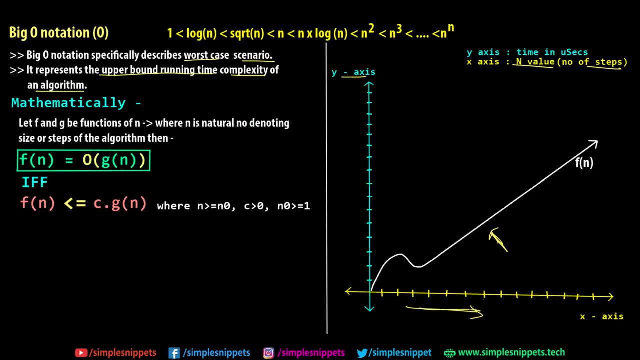 can be 10, 20, 000 and so on and so forth. as this n value increases, the time taken also increases, in a linear way. it's a straight line, right? so this function is a linear function and that's why it is known as linear time complexity. so this is something that we already saw in the previous. 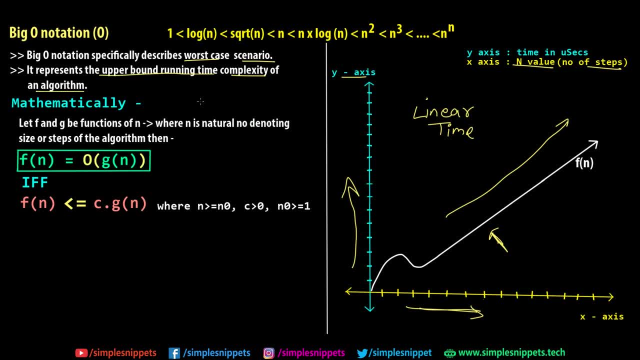 video. but how does it look like mathematically? because when we are doing algorithm analysis, obviously we want some numbers, we want some mathematical denotations, and that's what algorithm analysis is actually and that's where the functions come into picture. and these notations and 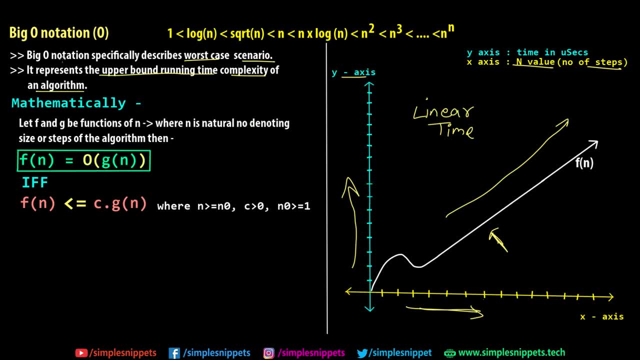 representations. so when you're specifically talking about big o notation, we are just representing the upper bound or the upper time limit, which is basically the worst case. right upper time is basically you saying that your algorithm will take maximum y minutes for x number of input. this is what. 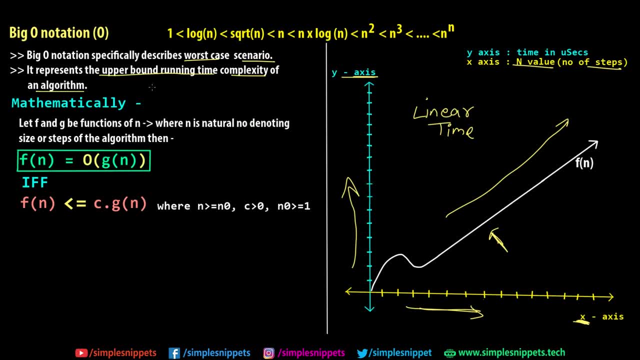 basically, you're trying to say that your algorithm will not go above this limit. so this is the worst case. that's what big o notation is. so how does it look like mathematically? so here we have let f and g be functions of n. so you can see f and g be functions of n. so you can see f and g be functions of n. 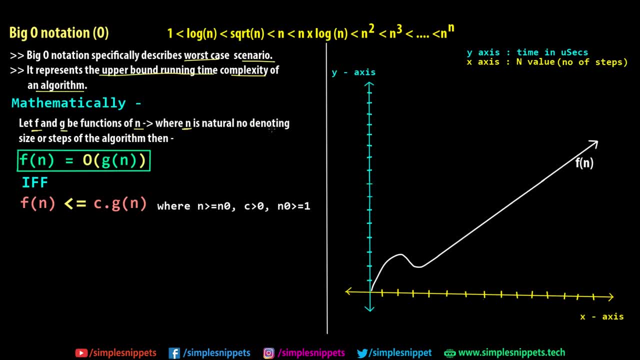 f of n over here, where n is a natural number denoting size or steps of the algorithm. so they are saying f of n is equal to big o of g of n if, and only if, f of n is less than equal to c. into g of n, where n is greater than n, naught, c is greater than 0 and n. 0 is greater than 1. now, obviously, 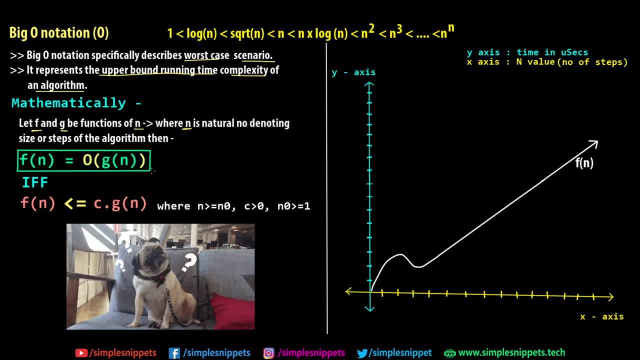 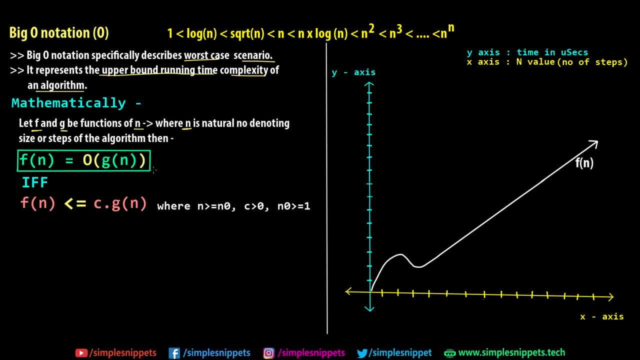 when you read it for the first time, you feel like what is this, what is this going on? because these mathematical notations are really tricky to understand at times when we see it at the first time. so let's try to break it down, let's try to understand this in a simple way. so this definition, 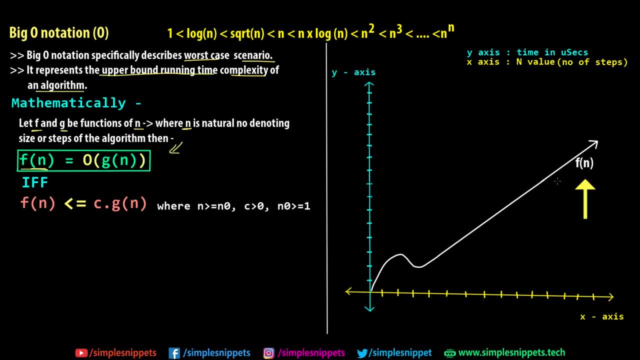 is basically saying that a function, f of n, which is this function- or you can see this behavior, linear behavior over here- f of n is equal to big o of g of n. so g of n is some other function. so we have f and g right. so this is some other function. so this g of n can be considered as 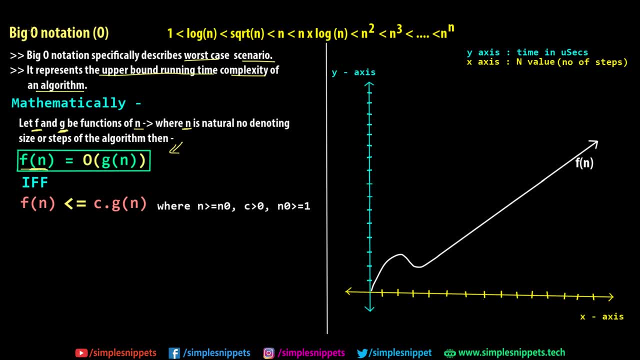 a upper limit of this function, f of n. that is what big o notation is, right, the upper bound. so it can be considered as a upper limit of this function. f of n, that is what big o notation is- can be considered as a upper bound or upper limit of f of n if, and only if, that is, only if. 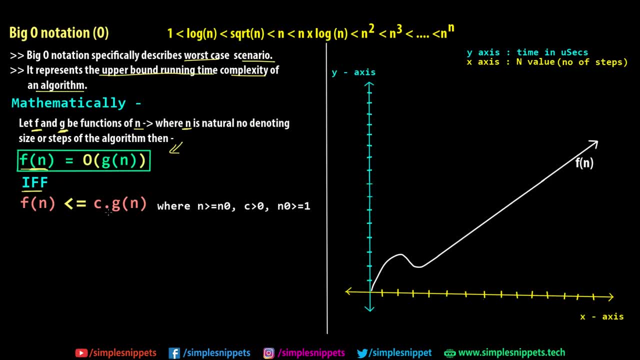 this function value is always less than or equal to c into g of n. so c is this constant, so it's a constant value and when you multiply it with this g of n function, it is always equal to the function or greater than the function. and n is obviously greater than n: 0. so after a particular n step, 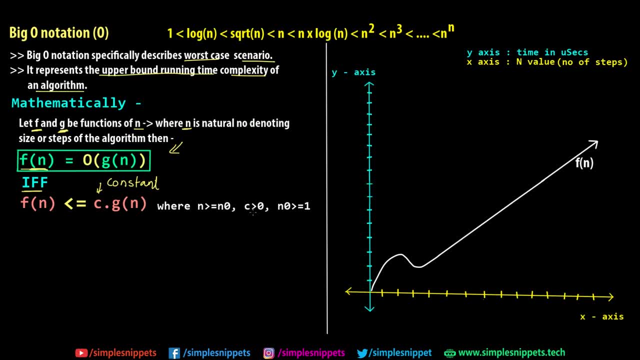 this equation holds true, or this condition holds true, and it states that f of n, which somehow has to be seen as ellos, will be greater than n. how does it count now as a moreıyı? well, let's assume f of n is greater than 1, right? so f of n is equal to 2n plus 3 hundred and a half, so you can add this f. 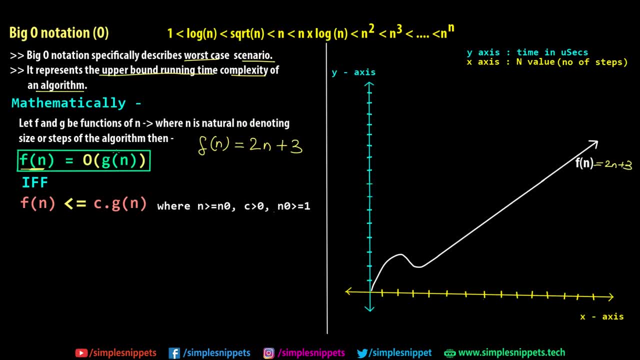 of n comes n plus 3. enter me, your answer is no. now let's just need to dig into some other 2n plus 3. let's take another function, g, of n, and let's say this is only equal to n. now what we want. 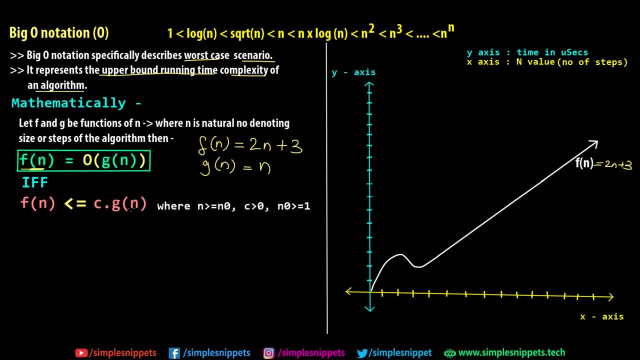 to prove is when we multiply a particular constant c into g of n, it is always greater than equal to f of n after a particular value, n, which is greater than n- 0. okay, so how do we go about this? so for g of n that is equal to n to be big O notation or to be considered as the upper bound of our 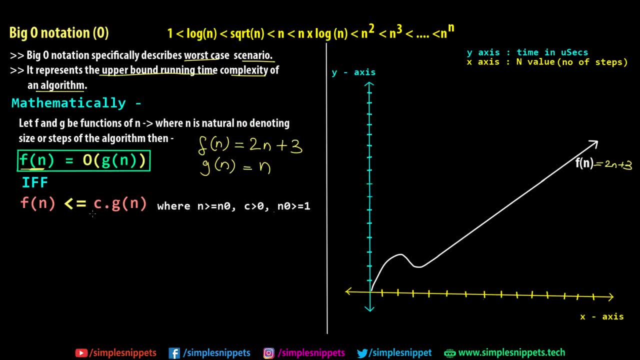 function 2n plus 3 what it has to be. it has to be multiplied with a constant c and it has to be always greater than or equal to f of n. so let me just write down 2n plus 3 over here. so lhs is f. 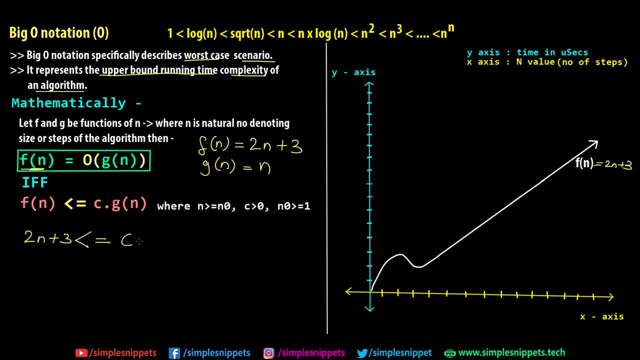 of n should be less than or equal to some value of c. into what is g of n? into n? okay, so let's consider c equals to 5, all right, and let's start off with n equals to 1, because, as i mentioned, n has to be some positive number, because n represents what? 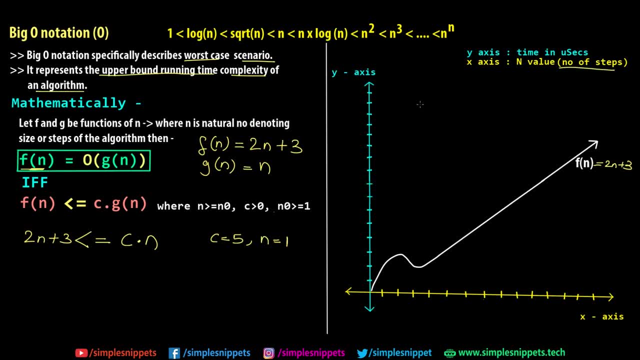 the number of steps in an algorithm, and obviously every algorithm has some number of steps. you cannot have a zero step algorithm, right? i mean, you can have a blank program or blank algorithm, but obviously it will not do anything. so we'll consider n equals to 1, so let's substitute these. 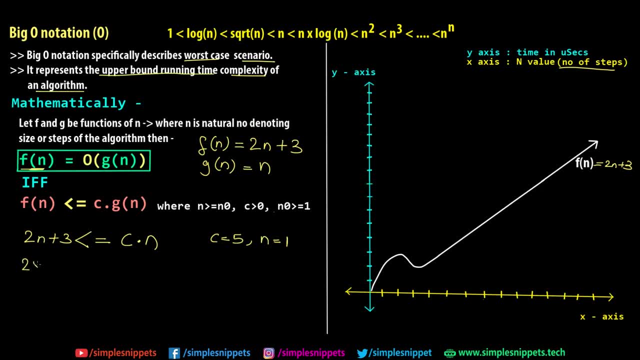 two values. so when we substitute n over here it would become 2 into 1, which is basically 2. so let's write 2 itself directly: 2 plus 3 should be less than equal to what is c 5. 5 into 1, now you. 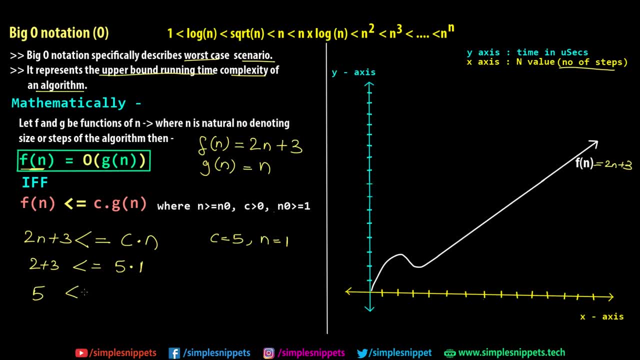 can see that we are getting 5 on the lhs, less than equal to 5 on the rhs. now, 5 is obviously not less than 5, but it is equal to 5, which means our condition is satisfied. so, on the graph, what will happen is we will have a additional line, or 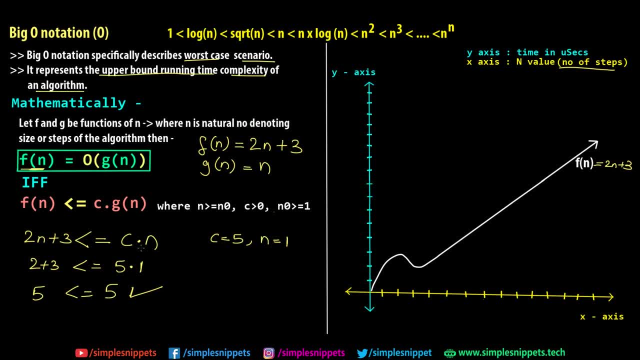 additional function which would represent c into g of n. okay, so c into g of n can be represented on the graph somewhere like this: okay, so this will represent c into g of n, provided c value is 5. okay, and for all values which are n equals to 1 or above n, or above 1, basically, so n to infinity. 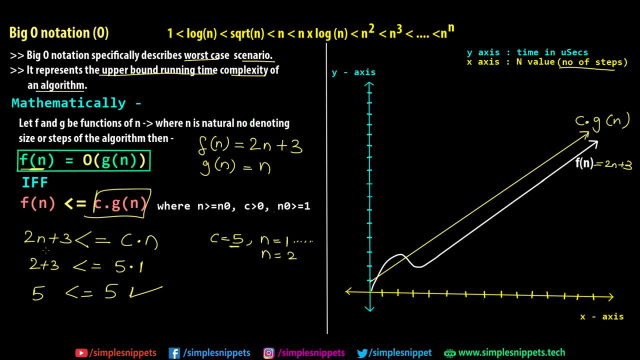 so if you say n equals to 2, what will happen if you substitute 2 over here? we will get 2 into 2, which is 4 plus 3, which is equal to 7, and on the rhs we will have substituting 2 over here, c is 5. 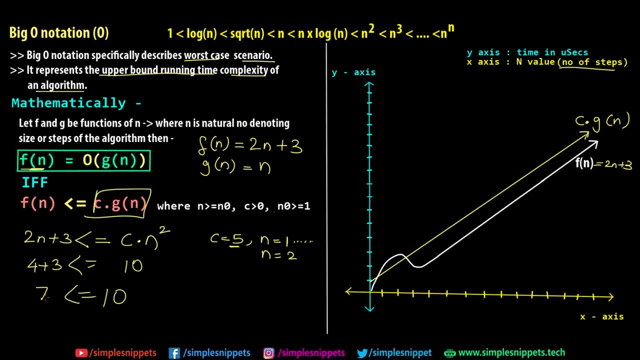 5 into 2, we will have 10, right? so obviously 7 is less than 10, which means, again, this statement is satisfied, right? so basically what we are saying is this: g of n is upper bound, or big O notation of f of n. so 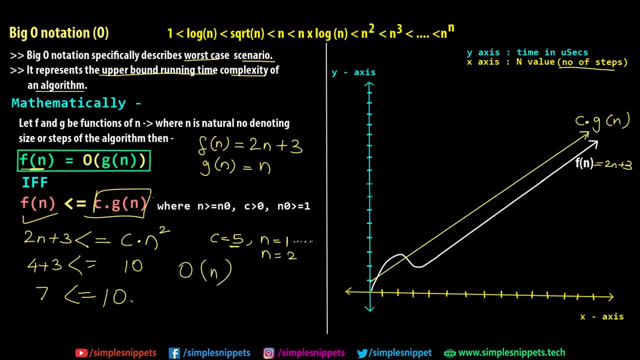 ultimately, we are left with o of n because g of n, what we assumed is n. right, we assume g of n as n, so this c is just a constant. so ultimately, our function 2n plus 3 has a big O notation of o of n. so this is what we proved and this is how the graph would look like and this: 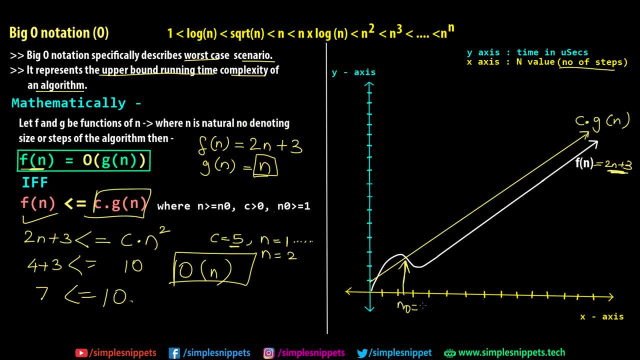 point is where n0 would be equal to 1. so after 1, this line, that is this yellow line, c into g of n will always be above our function f of n, 2n plus 3. if we take c as 4, let's assume the constant c as 4. 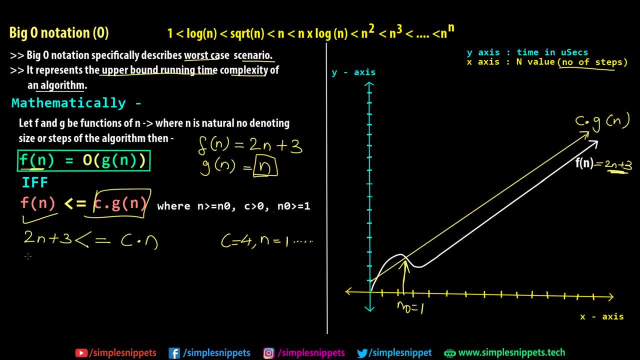 so c equal to 4 and n equals to 1. so now, if i substitute n as 1, so this lhs would be 5. less than equal to c is 4 and n is 1, so 4 into 1, 4.. So now four is obviously not greater than equal to five. you know, five is not less. 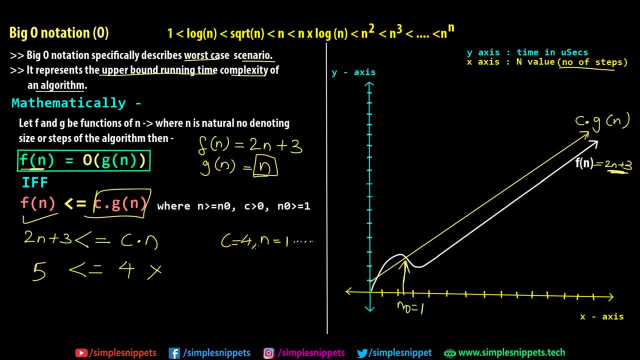 than four. right, So now the condition will become false. But what if we increase the n value to two? So now let's substitute these same values. So when I say n equals to two and c equals to four, so n is now two. okay, So two into two is four plus three, which. 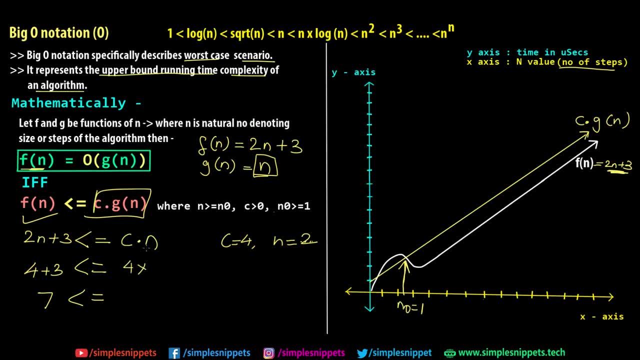 is seven, And on the RHS c is four. four into n is now two. four, twos are eight. So now we have eight, which is greater than or equal to seven. it is actually greater than seven, right. So now the condition is true, which means when the c value is four, the n value 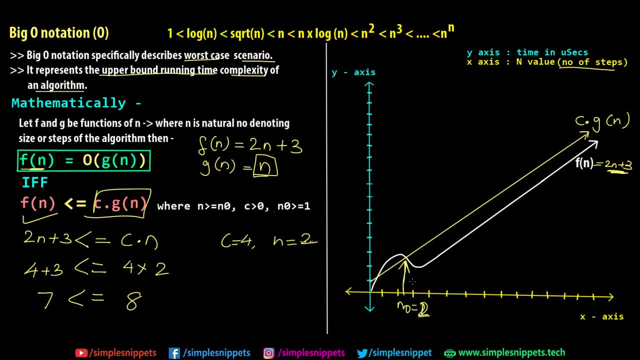 has to be two. So now n zero would be two. So after every value of n which is greater than n, zero, so n zero now has become two. So for every value of n which is greater than two, our c into g of n will always be greater than our f of n, right? So that is. 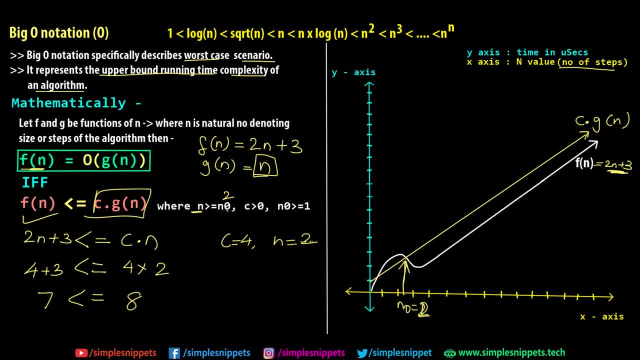 what n zero denotes. So the n zero denotes the value of n. It denotes that point after which our upper limit is always going to be upper, basically, and it is always going to be above our function. Over here, it is below the function, right. 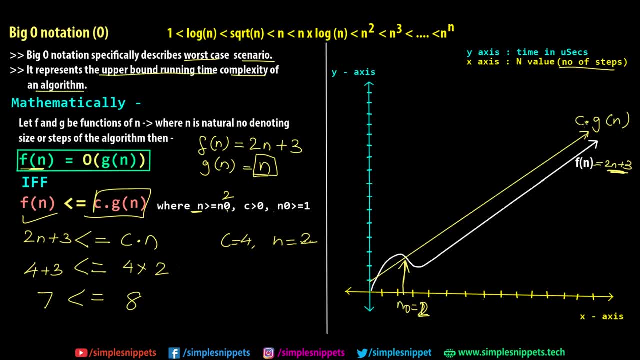 You can see the white curve is above, but after this point c into g of n is always going to be above f of n. So this basically proves that this g of n, whose value actually is n, is basically the upper limit, that is, is basically the big O notation for our function. 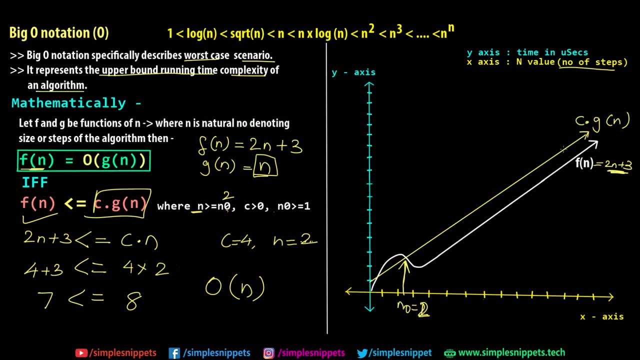 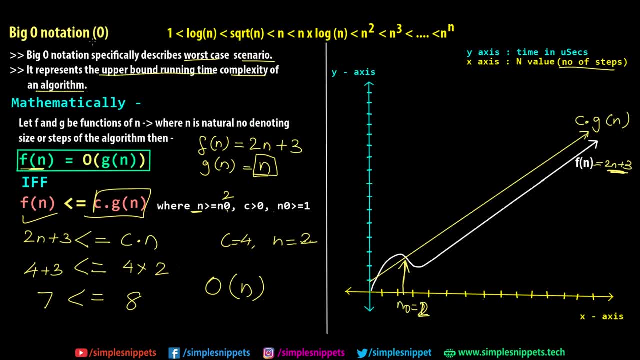 limit. Once we find the big O notation or upper limit, we can see that this two n plus three will always follow this behavior. Now, big O of n is usually denoted as linear time, So as the number of steps in the algorithm increase or the number of input size increases. 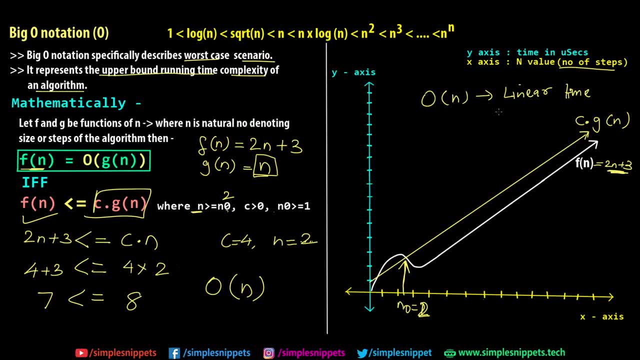 the time will also increase in a linear way. It will not grow exponentially. Now we can also bound. Okay, We can also consider g of n as n square. Let's see how that would look like. So now, what if we take g of n as n square? Okay, So this is basically quadratic time, And now we will. 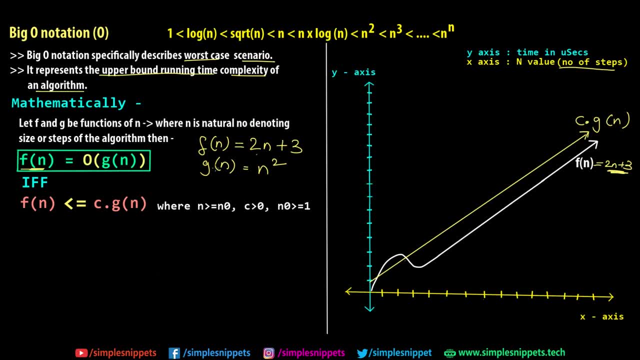 again take this f of n as same. So for g of n, which is n square, to be big O notation or upper bound of our original function f of n, it has to again satisfy this condition. We have to have a constant which has to be multiplied with g of n. So let's again write: 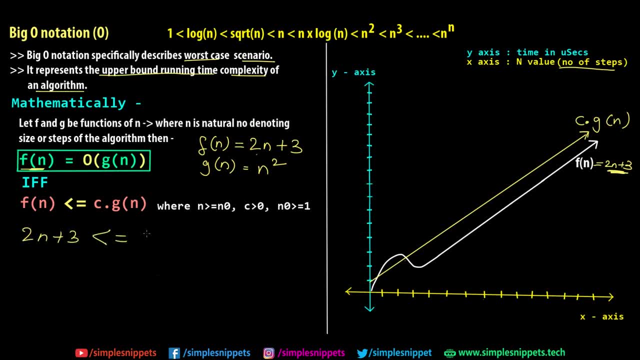 them to n plus three. So g of n should be less than or equal to c into our g of n, And in this case g of n is basically n square. Now let's assume c equals to one And let's start off with n. 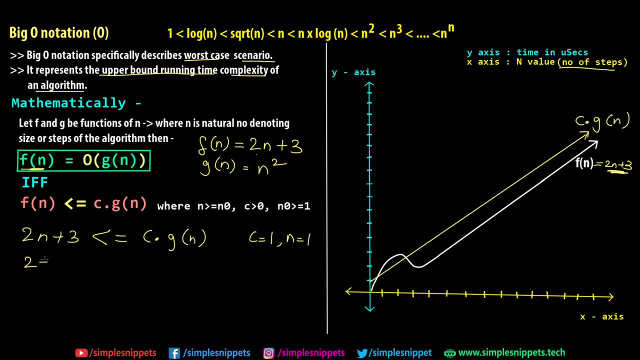 value as one. So, substituting n as one, we have two plus three, which is equal to five on the LHS. What is g of n? n square? So n is one initially, So one square is one. C is also one. We have one over here. So this is not true, right? Two plus three, or basically: 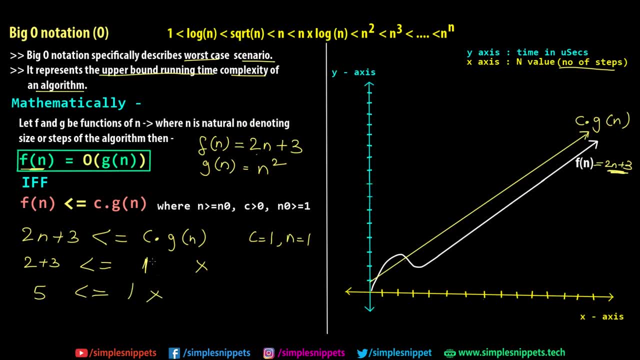 five. Okay, So g of n is equal to one. Okay, Let's increment the n. Let's now take n as two. Now, when n becomes two, we have two into two is four, two into n, right, So this is four plus three. 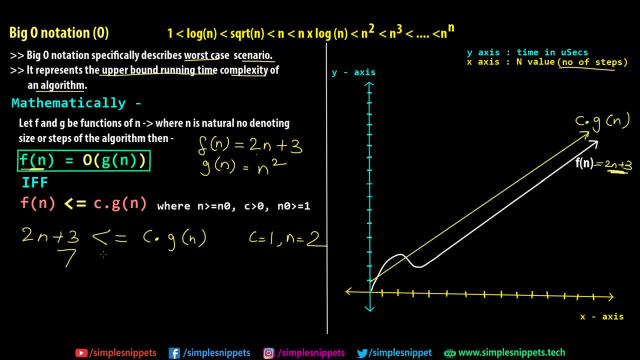 which is basically seven. Let me just write it over here: itself Seven. And on the RHS we have n square, So n is two, So it becomes four, and c is one only. So still, four is not greater than seven, or seven is not less than four. So again, this is also false. Let's 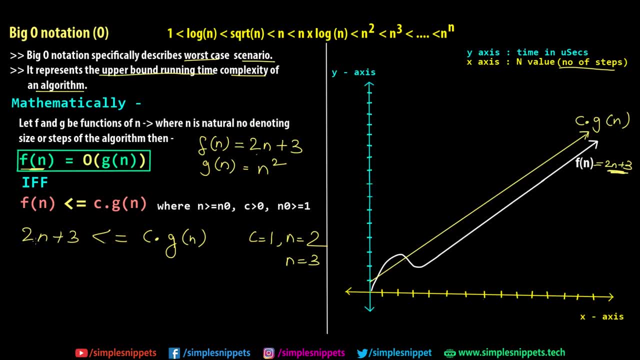 take n equals to three, Now n is three. two into three, six plus three, nine less than equal to c is one. So one into g of n is n square basically. Now we substitute three over here, So three square is nine. So now you can see: nine is equal to nine, So now 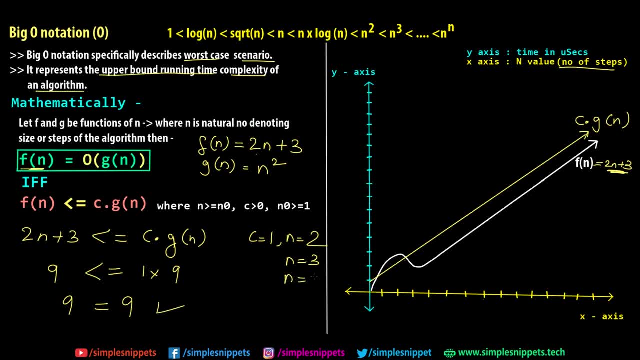 it became true. And now, if you substitute four as n, this, this side will be 16, right, So let's do that. Let's take n equals to four. What is two into four, eight eight plus three is 11, is 11 less than equal to. when substituting four at n, square, it becomes 16.. Yes, Now 16. 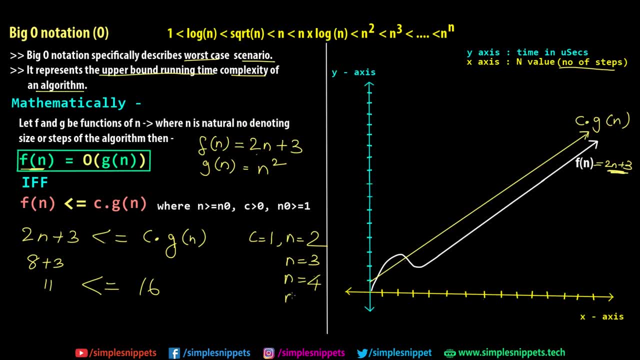 is greater than equal to 11.. It is actually greater, which means that now, as the n values increase after three, all the values of n will satisfy this condition. So this point over here is n zero point which is equal to three. So for n which is greater than, 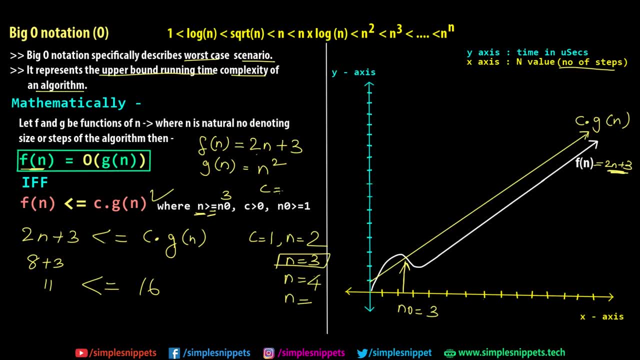 three or equal to three, Which is greater than zero. Obviously c is greater than zero. All the values will satisfy this condition, which means that we can conclude that this new g of n, which is n square, is also big O notation is also upper bound for our original function to n plus one. So we 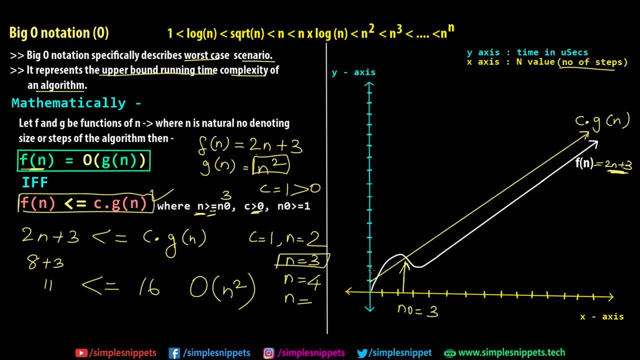 can also say n square, and n square essentially would look something like this on the graph: It is basically exponential, It is a curve, So this would be c into g of n square, basically, And originally c. we were assuming c as five, So let's keep this five and this is basically one. So now, 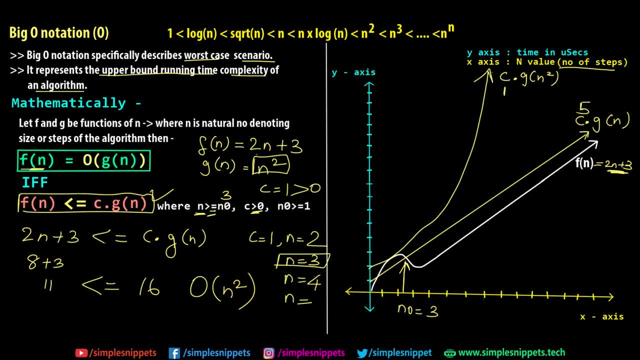 you will say, okay, so even this n square is also upper limit or can also be considered as the upper bound for this original function f of n, which is also true. But when we actually try to find out the big O notation, what we have to do is we have to find the closest. 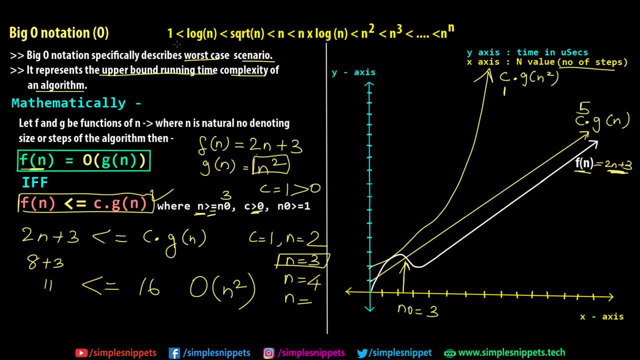 one which matches the f of n. So over here I have a chart which basically denotes the time complexities in their mathematical terms, in a particular order. So this one represents constant time. Then we have log n. So these are all behaviors on the graph. Okay, so they all look different on the graph. We have n over here which is 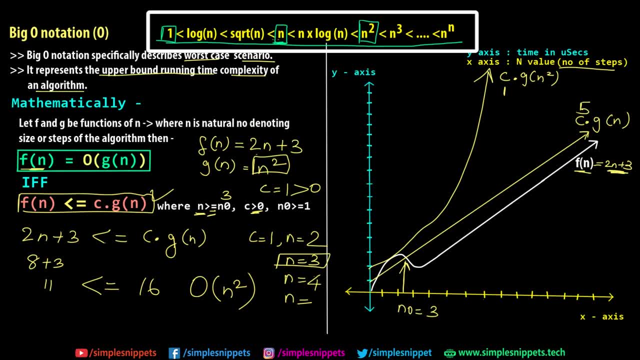 linear and we have n square over here. So n square, you can see, obviously is greater than n. it is on the right hand side. Now we just proved that n is also an upper limit for our original function to n plus one. So we have to take the closest one, which is, which is actually n only. So this is O of. 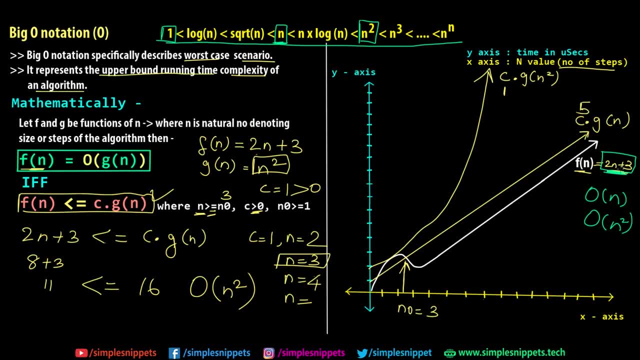 n. Okay, square for this, two n plus one, But, as I mentioned, we have to take the closest one. Okay, So this was big O notation or the worst case scenario. Now let's see what is the best case scenario, which is the big Omega notation. Okay, So let's see what big Omega notation. 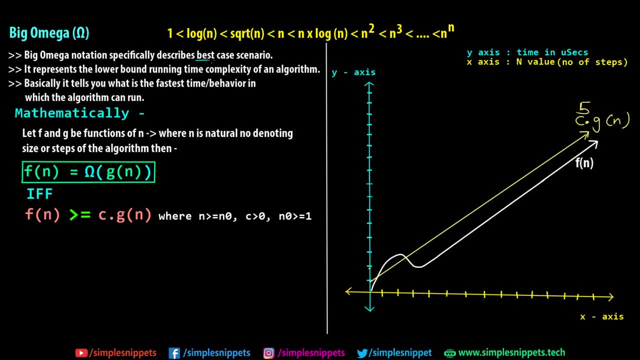 is So. big Omega notation specifically describes the best case scenario. Now it represents the lower bound running time complexity of an algorithm. So it's basically just opposite to big O, because big O was the worst case. Big Omega is represented by this Omega sign. 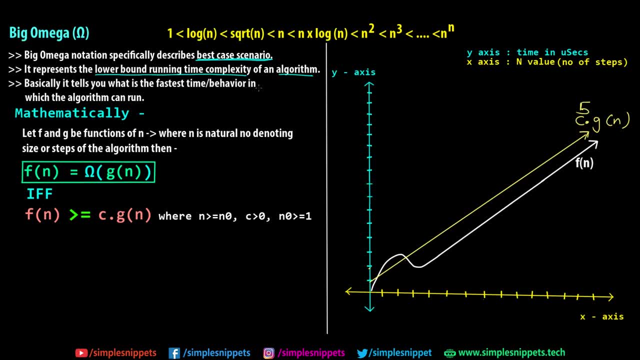 gives the best case. So basically, it tells you what is the fastest time, behavior, fastest time or behavior, basically, in which the algorithm can run. Okay, Big O was saying what is the slowest time or what is the worst time. Big Omega will tell us what is the fastest your. 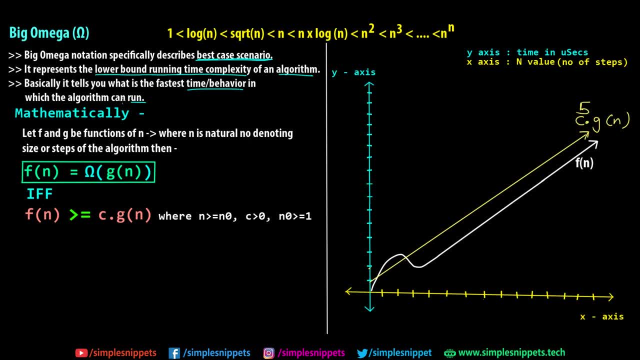 algorithm can run given a particular set of input or size of input. So how does it look like mathematically? Because obviously we need some numbers, We need some equations, because you're dealing with asymptotic analysis, which is mathematical representations. So again we have some condition, So we have 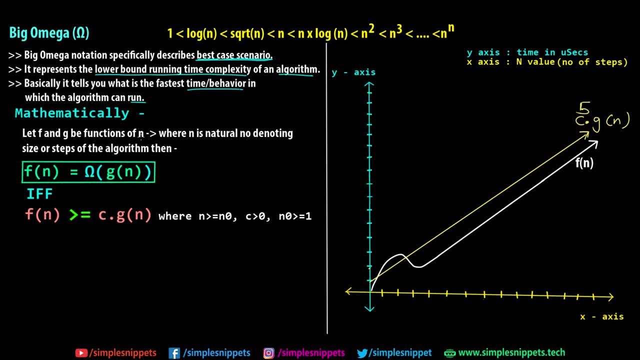 let f and g be functions of n, just like we did for big Omega, where n is natural number denoting the size or steps of algorithm. Now a function f of n is equal to big Omega of g of n. So we have another function, g of. 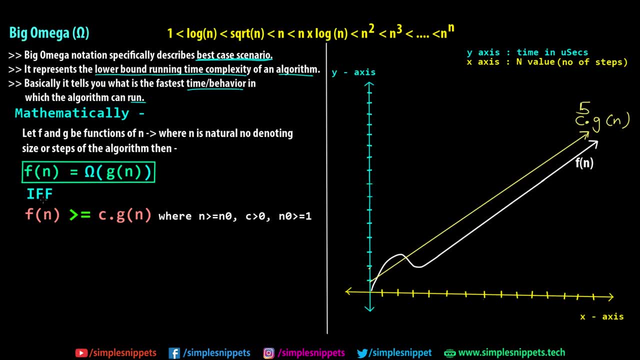 n, which can be considered as big Omega of f of n, if, and only if, our function f of n is always greater than equal to this g of n, which is multiplied by a constant value, where, again, n is greater than a certain value of n, not c is greater than zero and n not. 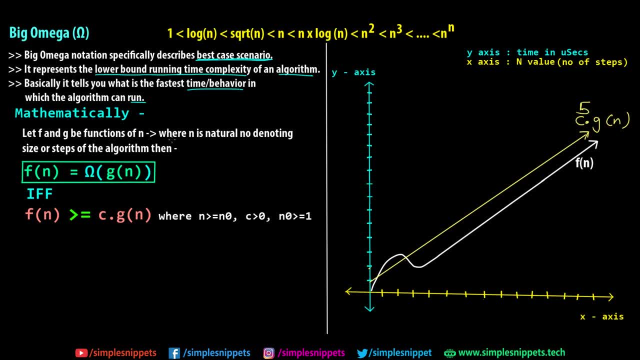 is greater than or equal to one. Okay, so this essentially is giving us the lower limit and obviously, just by reading the mathematical conditions over here and these equations, it doesn't make any sense, Right? So let's take the same example. Let's again denote. 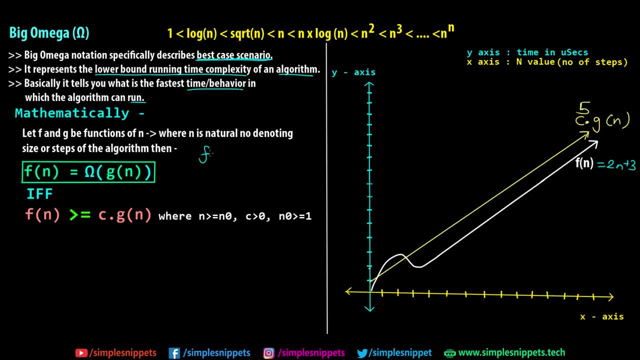 f of n as two and plus three. Okay, so let's consider f of n as two and plus three and 2n plus 3.. Now again, we will take g of n also, and now g of n will represent it as the same. 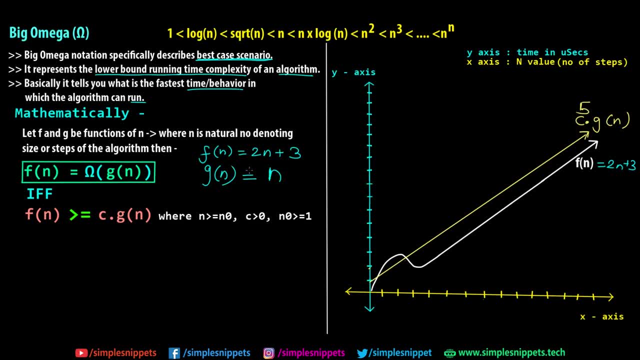 one that we did in the previous one, which is taken by n. So for g of n to be big omega of our f of n, our original function f of n, it has to follow this or it has to satisfy this condition. So f of n is 2n plus 3.. 2n plus 3 has to be always greater than or equal. 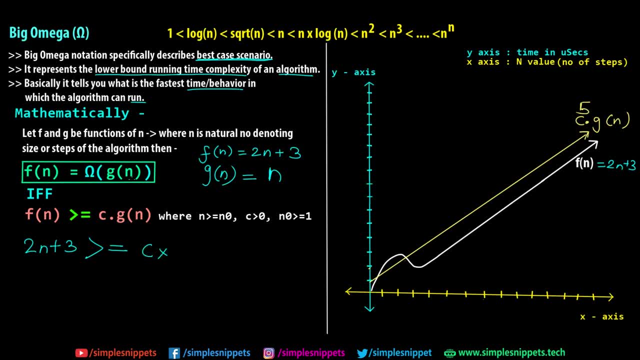 to a constant c multiplied by the assumed g of n, which is n. Now let's take: c equals to 1 and just by looking at it, when we substitute 1 over here, it would be 2n plus 3 greater than or equal to n. Now, obviously, just by looking at this equation itself, you can say: 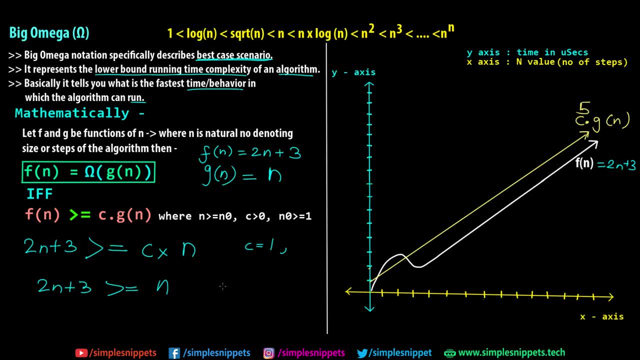 that 2n plus 3 is always going to be greater than or equal to n for any value of n starting from 1, right, If n is equal to 1, we substitute 1 over here. we substitute 1 over here it. 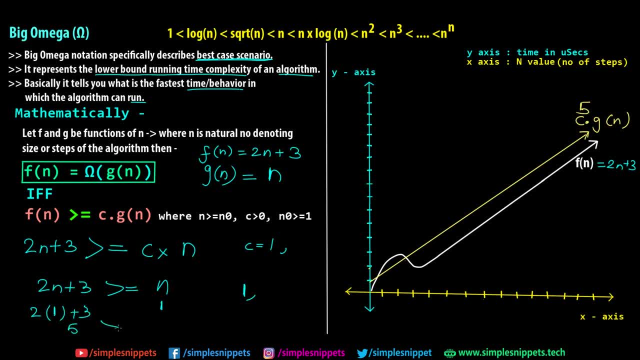 would be 2 into 1 plus 3.. So obviously it would be 5, which is greater than 1.. If you substitute 2 also, this would be 2 and this would be 2.. We will multiply 2 into 2, 4, 4 plus 3 is 7.. So 7 would be. 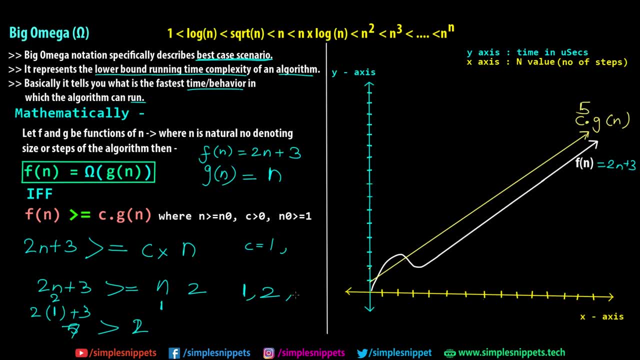 obviously greater than 2, or you substitute any value of positive integer of n, that is, the steps number. This equation is always going to be satisfied, which means basically, we already have proved that this g of n can be considered as big omega of our function. 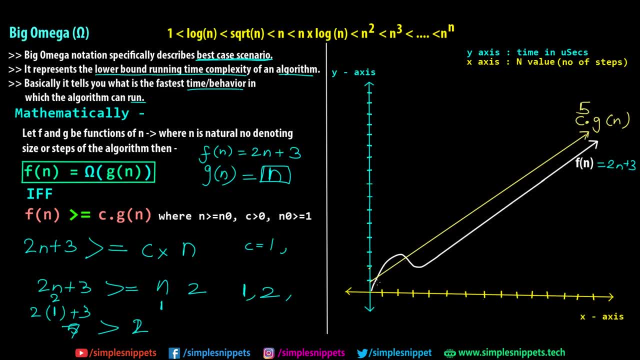 2n plus 1.. So how does that look like? So the way it would look like on the graph, it would be something like this: It would be again, c into g of n. So this is that, c into g of n, and 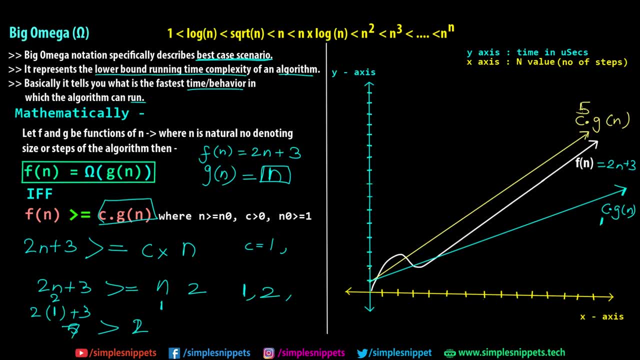 this time c value is 1, okay And not 5.. When we take c value as 5, it would be above this function, but when we are taking c as 1,, it is always going to be below the g of n and 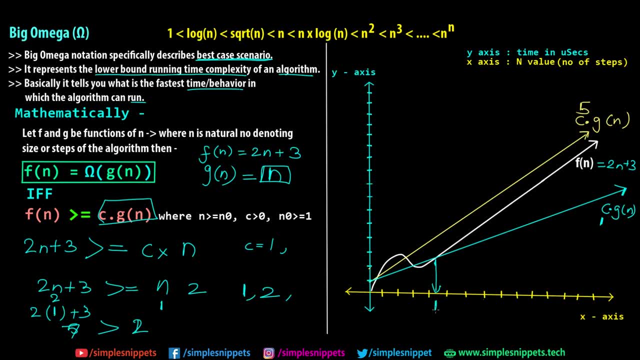 this n0 value is basically going to start from 1 itself, So this is n0.. So for all values of n which are greater than or equal to 1, this equation holds true when we have g of n as n and f of n as 2n plus 3.. Hence we can say that this: 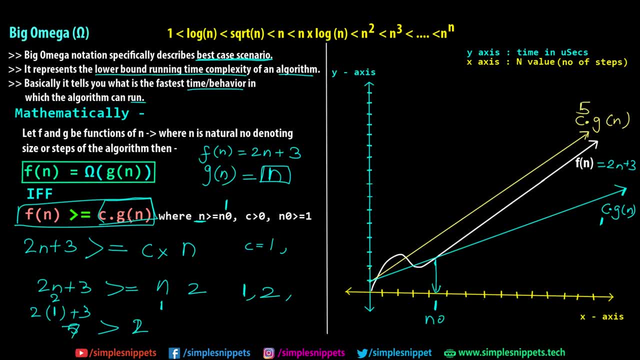 g of n, which is equal to n, is big omega of f of n. okay, So we can say big omega of n because g of n is n, and we can say that this is the lower bound for this function, which is the lower limit. So this was big omega, which gives us the 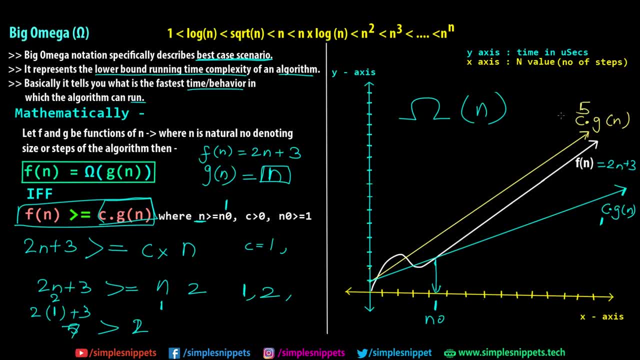 fastest time. Generally we are not really interested more in the fastest time. We are more interested in the worst case scenario, because we want to test our algorithms for larger inputs and we want to see what is the worst time it will take. Only then we can. 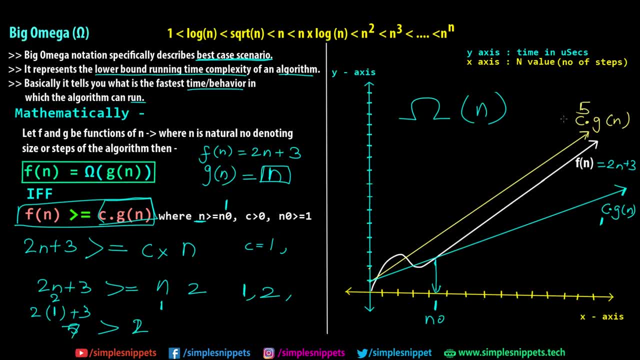 make other decisions in the further process. So this was big omega. So now let's see the last one, that is, theta, or big theta notation. What is that? Also, before going to the big theta notation again, we just found out that the big omega. 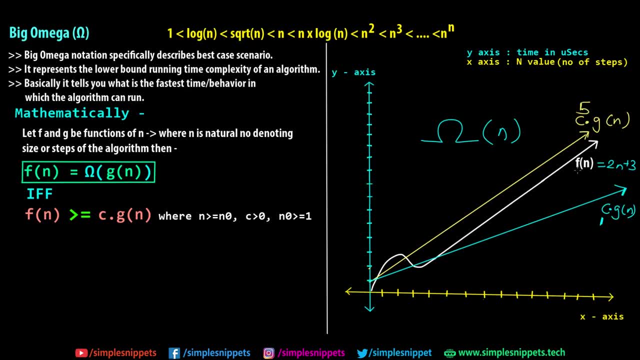 is big omega of n for this given function, but it can also be something which is lower than n. Now in this map or in this hierarchy, you can see that what is lower than n, square root of n, log n and constant time. So constant time would look something like this. It would: 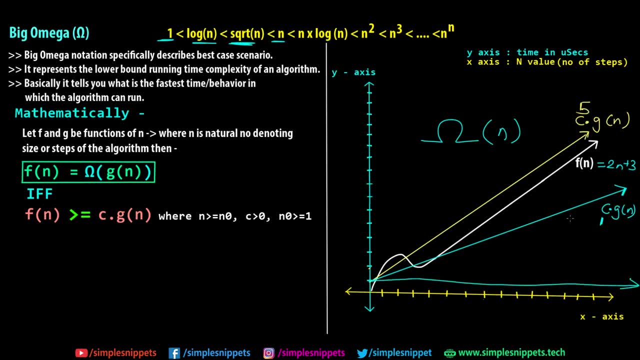 be a constant straight line, and even this can be considered as the lower bound for f of n, right, Because you can see it is never going to be above our f of n. But again, we have to take the closest one. The closest one to our original f of n. and the closest one to the original f of n is: 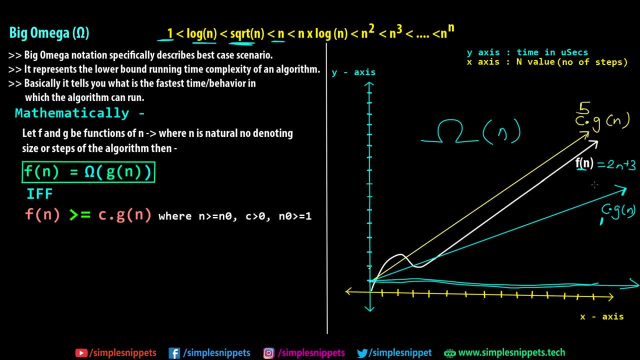 g of n, which is n only. So we have to always take the tightest bound to get the closest match. Okay, Be it on the upper bound, or be it on the lower bound, Okay, so let's move on to the last notation. So the last notation is known as big theta notation and big theta. 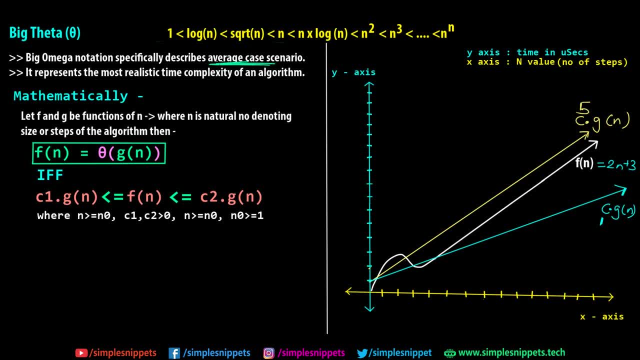 notation specifically describes the average case scenario. So basically, it gives us the most realistic time complexity of an algorithm, Because not every algorithm is the most realistic. So basically it gives us the most realistic time complexity of an algorithm, because not every time your algorithm will perform the worst, or not every time the algorithm will 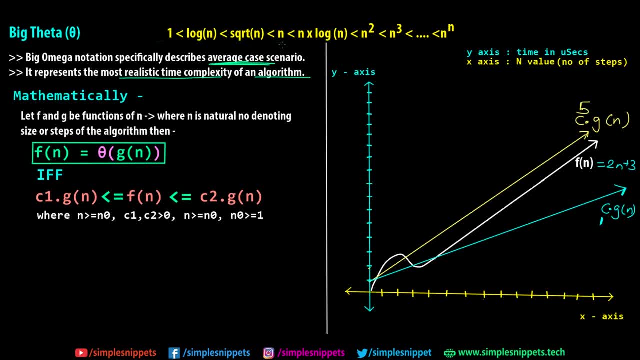 perform the best right in real world scenarios, your algorithm will fluctuate from the worst to the best ride, So we need our center value, we need an average case, and that's where big Theta comes into picture, and usually big theta is used when the best case and the worst case. 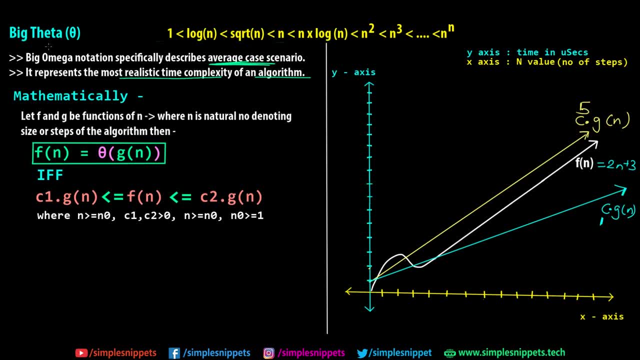 of certain algorithms is the same. Okay, that's when the big theta is used. So for some algorithms, the best case and worst case are different. For some algorithms, the best case and worst case others same. So you'll see that when we actually move ahead in this tutorial series, when we 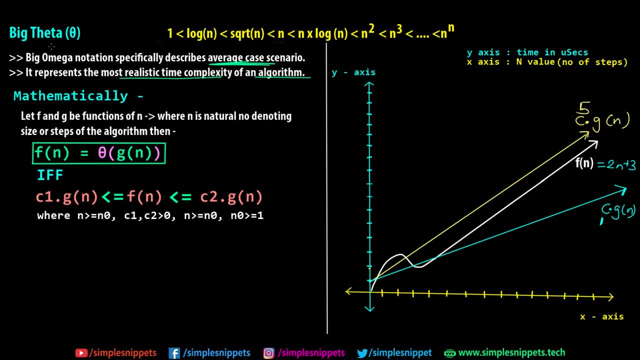 actually calculate these different notations for individual algorithms. if you want that, you can let me know in the comments And we can do that for individual algorithms. Okay, But mathematically this is how the big theta looks like. So let f and g again be functions. 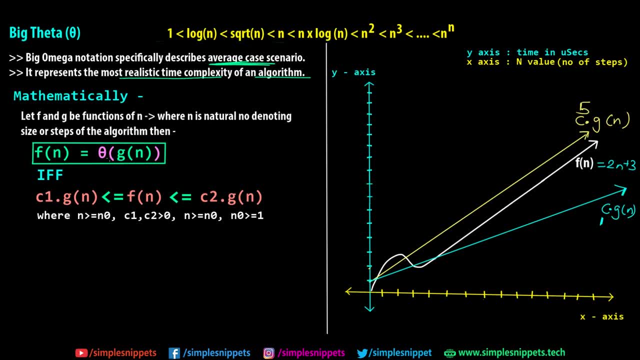 of n, where n is a natural number. So this g of n can be considered as big theta of f of n, if, and only if, there exist two limits. So we have c1 into g of n, which is less than equal to f of n, but we have c2 into g of n, which is greater than f of n. So you can. 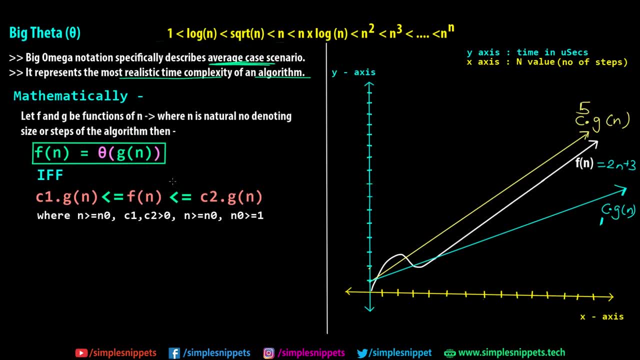 see, we are basically bounding the upper and lower limit over here And our original function is in between. So again, let's consider the same: f of n equals to two n plus one, and g of n to be considered as n. Now, just by looking at the graph itself, we actually have the 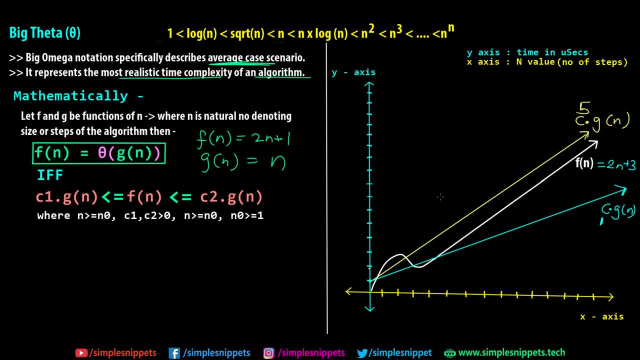 two values of c1 and c2, right. c1 would be this, the lower limit, because c1 into g of n should be less than or equal to f of n. So c1 has to be one and this has to be c2, right? So c2 has to be equal to five. So let's. 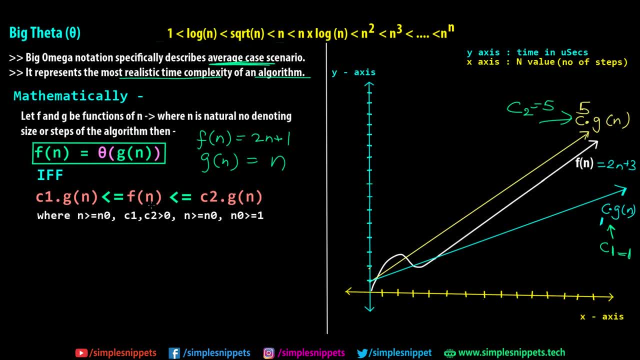 just substitute these values into our original equations over here. So in between we have two n plus. this is actually three and not one, So two n plus three. c1 is one and g of n is n, So one into n. it should be less than equal to two n plus three and two n plus. 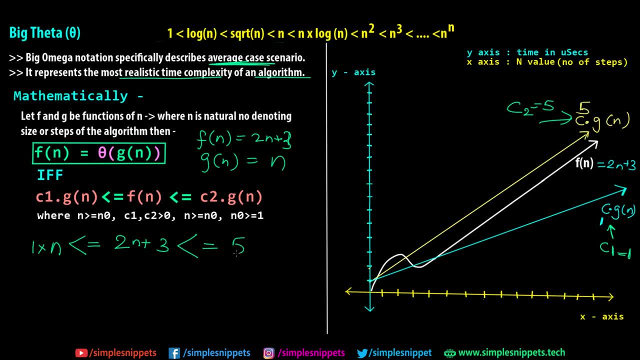 three should be less than equal to, and c2 is what? Five. So five into n. So if we substitute n equals to one, let's start with n equals to one, So this would be one which is less than equal to two into one is two plus three is five. 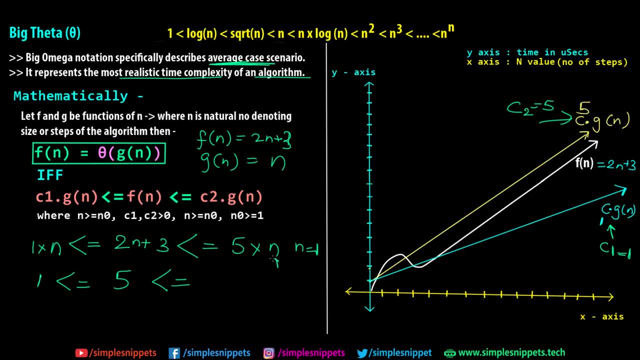 which is less than equal to. when we substitute one over here, five into one will become five, So this is true. So if we have n equals to two, again, if we substitute these same values, so one into two, less than equal to, again, we are substituting two over here, So two. 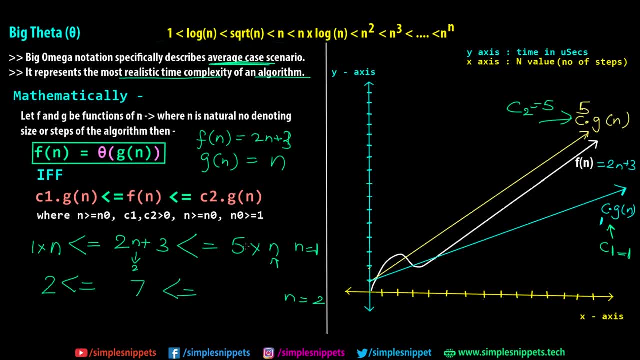 into two is four plus three is seven, which is less than equal to five. into two is 10.. So for this also it is true. So hence we can say that g of n is theta of f of n. Okay, So for this function, f of n equals to two, n plus three. the big theta notation is n. 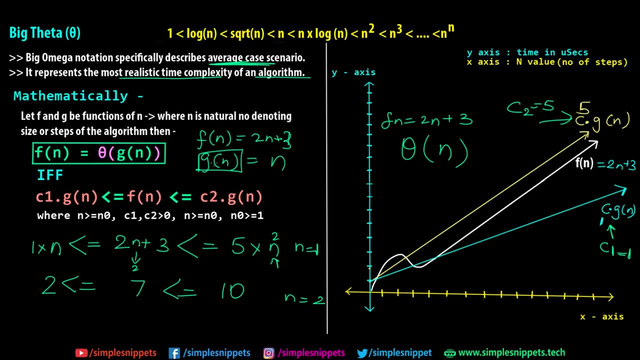 So theta of n, because g of n is n right, And we are saying this: g of n is considered as f of n When these conditions match and these are matching over here. we've just proved it mathematically. So this was the average case scenario. Okay, So this basically was: 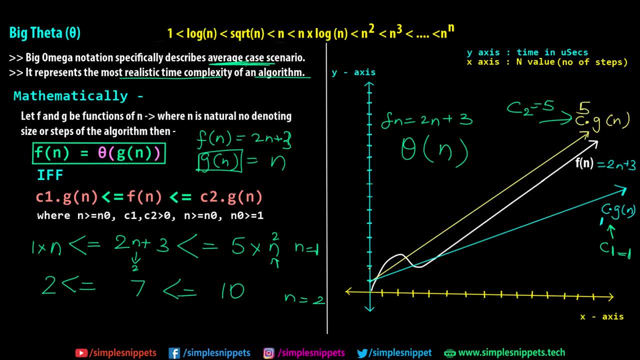 the average case scenario, which gives us the realistic time: the average case scenario. Okay, So these were the three different notations, And one last question that you might have in your mind is: how does it look like in real world scenarios And why do we have three? 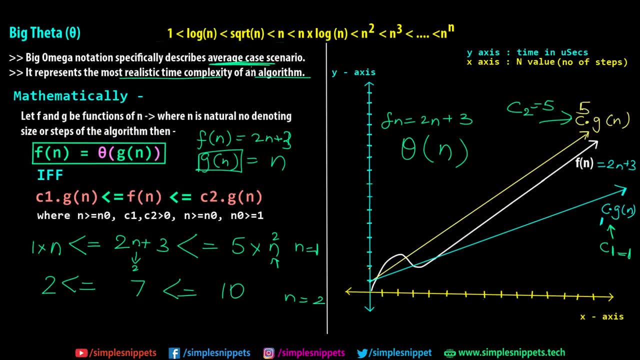 different cases, And I did mention that some algorithms have different best case and different worst case, So that's why we have to calculate them individually, And some of them don't have. So how does that really look like? Can we have an example? 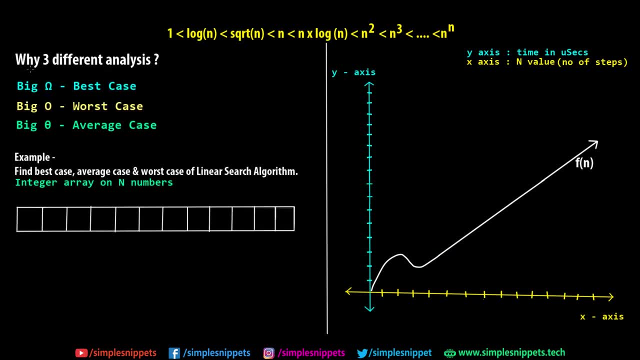 So let's see an example. So last question that we have is: why three different analysis? Let's take an example. By now we've understood that big omega is the best case, Big O is the worst case and big theta is the average case. So here's an example We have to find. 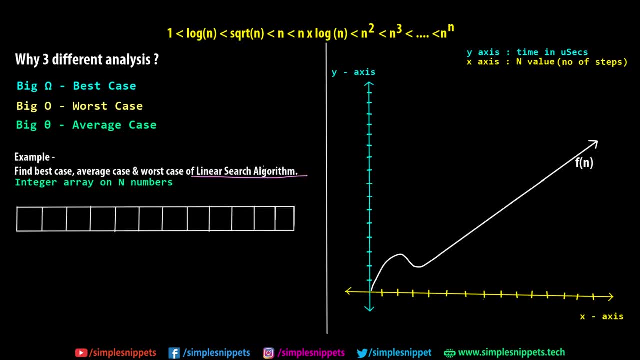 the best case, average case and worst case of linear search algorithm. Now, if you don't know what linear search is, we've already talked about it in this data structure series. You can check out the entire playlist course. You'll find the linear search. We also have written program for it And basically we have 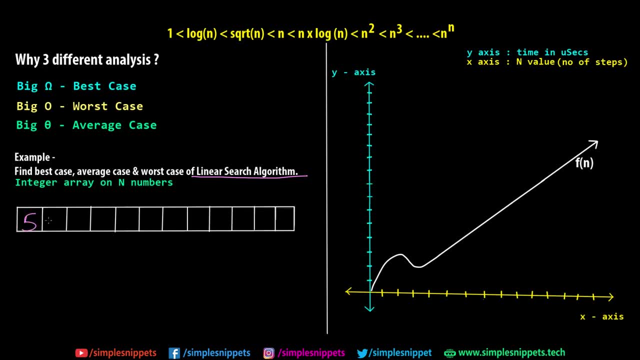 an integer array of n numbers. Let's have 5,, 4,, 1,, 7,, 20,, 11,, dot, dot, dot, so on and so forth, And at the last we have a hundred. Okay, This is the nth term. This is the zeroth. 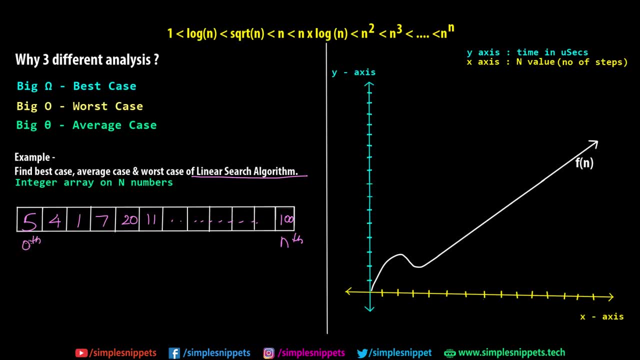 or basically the first term Array index starts from zero, right. So our linear search basically will start from this location. It will move on to the next, move on to the next till we find the match. So let's say we want to find out the value is equal to five. So when you want to find out the value, 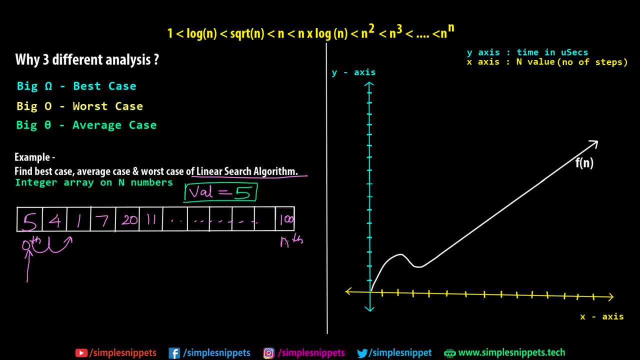 equal to five. you can see, if you see this array which has n elements, the value is at the very start only at the zeroth index. So in the loop, when we are searching through the array, it will take only one single iteration to find our match and then our algorithm will. 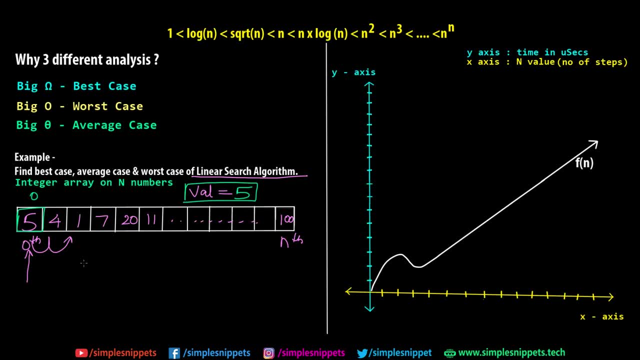 exit. So this, basically, is the best case, right. So the linear search, the best case is constant time, essentially right. So you can say big omega of one itself, because in the very first iteration we got our output and the algorithm stopped. but not everybody's as lucky as us, right? So that's when the worst case comes. 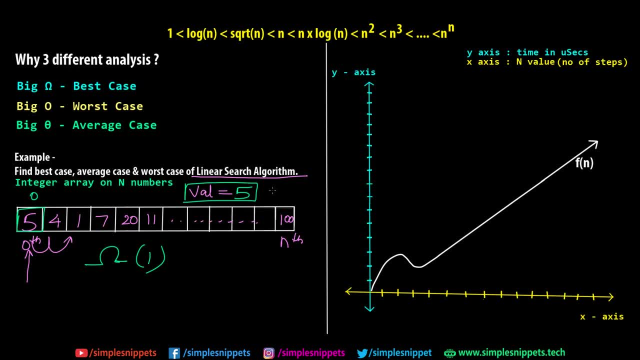 into picture. What if the value that you want to search is not five? the value that you want to search is equal to a hundred, So it's not five, it's equal to a hundred. Now, if we want to search for a hundred, we already know the hundred is at the last position. 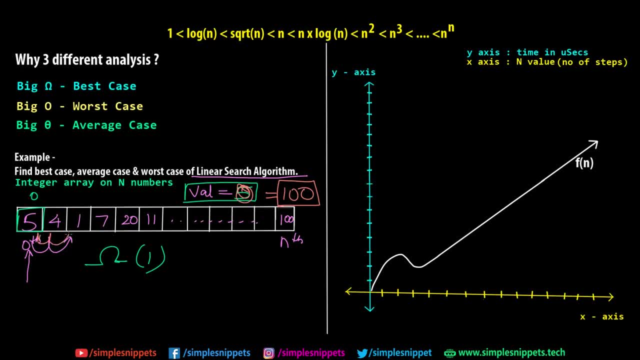 So our search will start from zero, It will go to next, It would go to next, It would go to next, It would go to the next, and it would have n iterations, because a hundred is the nth item. So after n iterations, finally it will find a match. So you can see our algorithm. 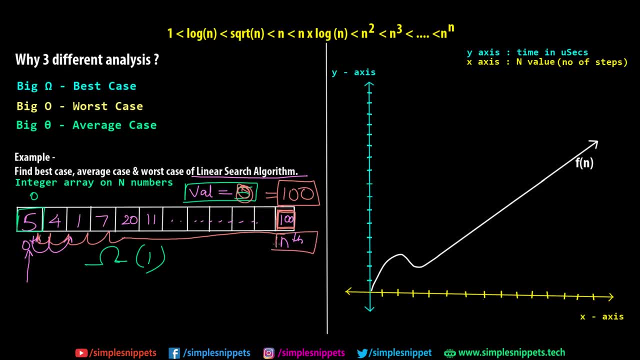 had to run for n times. Now, this n can be thousand, also right. We can have set of thousand elements, or size of our array can be thousand, It can be 10,000. It can be lakh, And if that element is at the end of the array it will have to run for all the different locations. 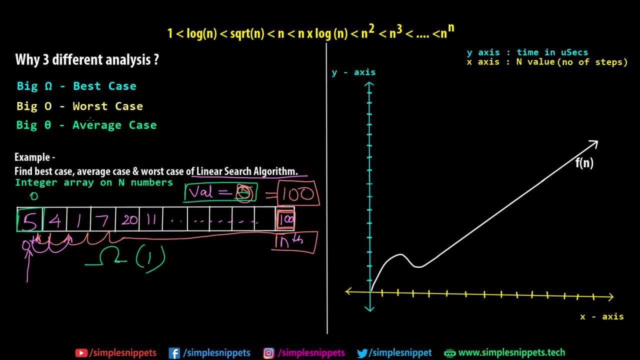 and you'd have to search for all the different locations. So that is the worst case. So the worst case can be considered as off n right Because it is at the end of the array list. So you can see we have two different time complexities. The best case is constant time. 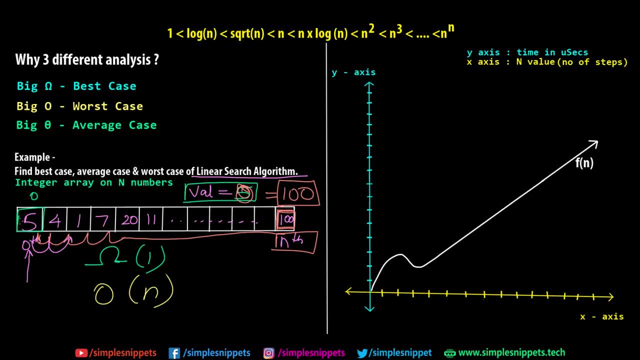 one, because our element to be found out was found out at the very first when we want to find out fi, but when we want to find out a hundred it is at the very last, so that's the worst case case. so it has to iterate through n elements. so O is n, so what would be the average case? now the? 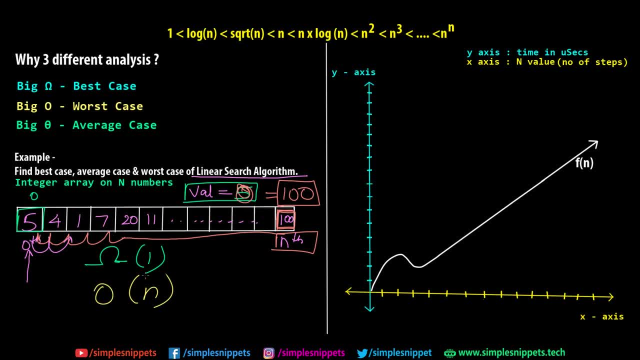 average case can be obviously easily understood by taking a mean of them. so mean point will be the midpoint. so it would be n by 2, right? so essentially it would be something like theta of n by 2. but when we consider time complexities in a asymptotic notation we do not consider. 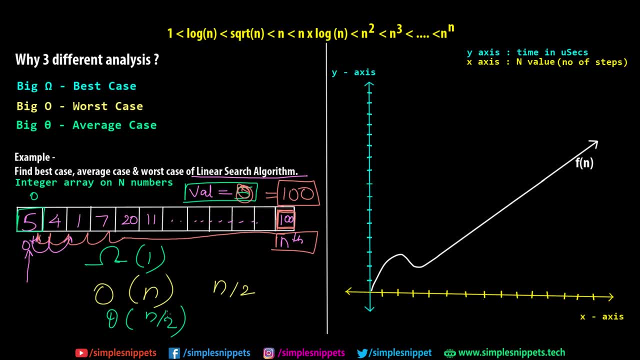 constant values. so we eliminate all the numbers, we only keep the variables. so this would also be theta of n only. so the average time and the worst time pretty much matches each other, but the best case you can see is one. so that's what the difference is all about. so this is the omega.